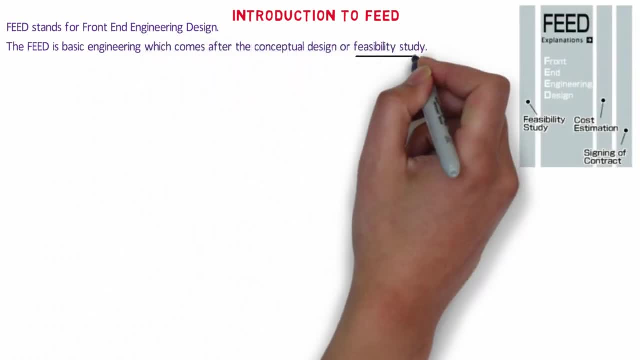 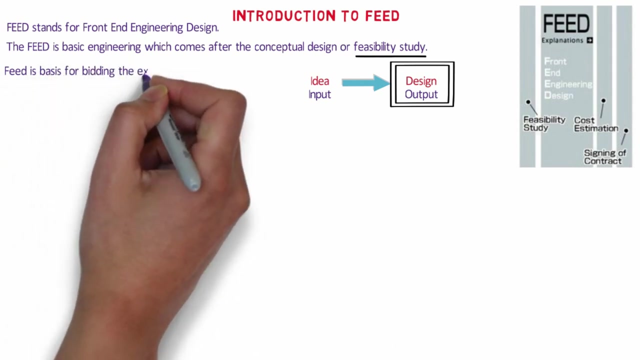 the conceptual design or feasibility study. The Front End Engineering Design is the process that take an idea and turn it into design. It consists of an input, which is an idea, and change into the current product, which we call output, final design or process. The FEED can be divided into separate packages covering different portion of the project. 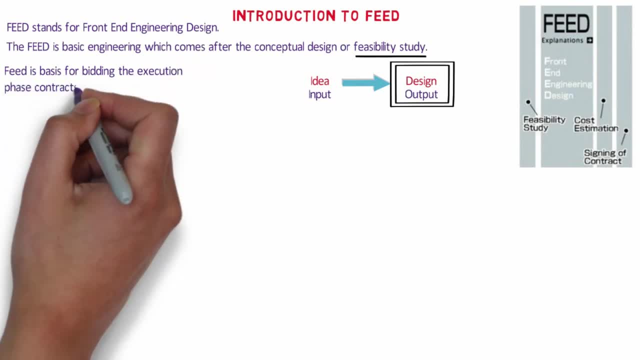 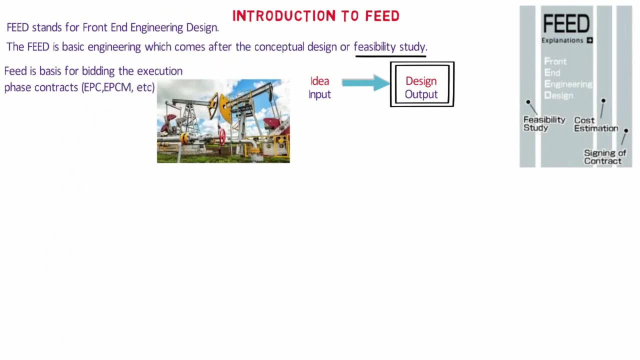 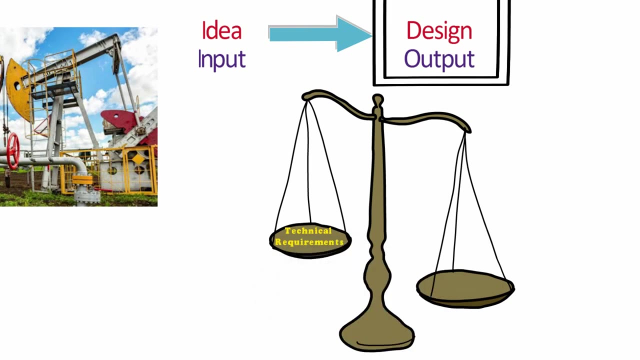 The FeED package is used as a basis for building the execution phase. contracts like EPC, EPCI, etc. FEED takes into account everything related to marketing the infrastructure or technology related to the project before actual steps are taken. The feed focuses on the technical requirements as well as rough investment costs of the project. 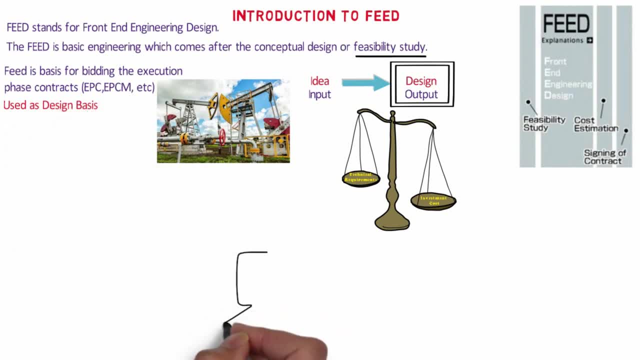 and are used for the design basis. Based on the extent of detailing and stage, feed can be defined as basic feed, intermediate feed or extended feed. We will explain the difference later. Feed shall reflect all the client project specific requirement so that significant changes. 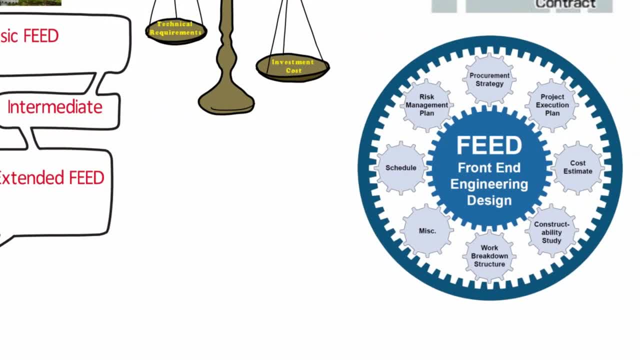 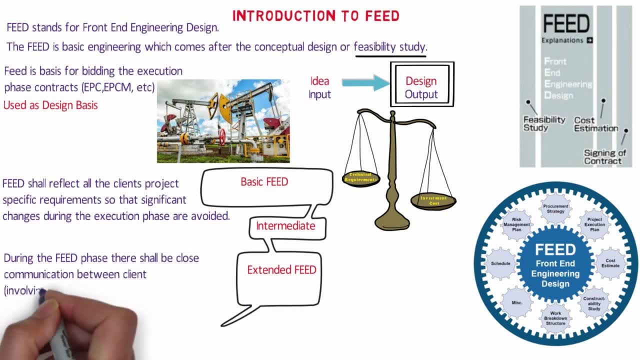 during the execution phase are avoided. During the feed phase, there shall be close communication between client, which should also involve the maintenance and operation team from the client side, and the feed contractor to work up the project specific requirement. The feasibility study evaluates the project's potential for success. 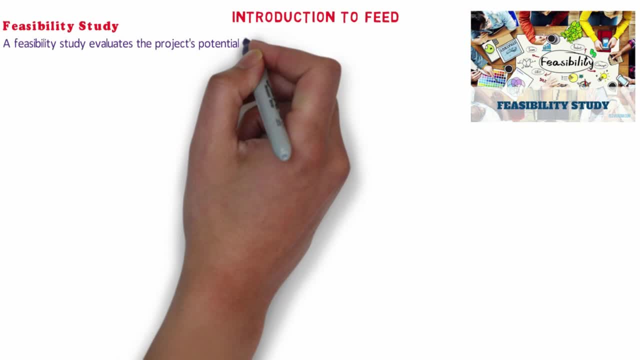 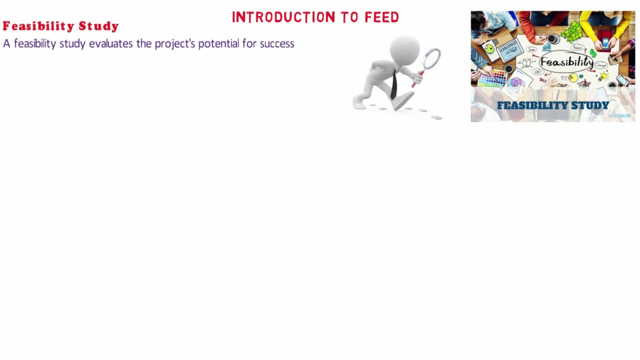 Analysis for the potential for the proposed project, which is based on extensive investigation and research, to support the process for decision making. Feasibility study is the starting point of the feed. Let's see what are the deliverable requirement for the feed. As I said, this video is only for the perspective of the piping. 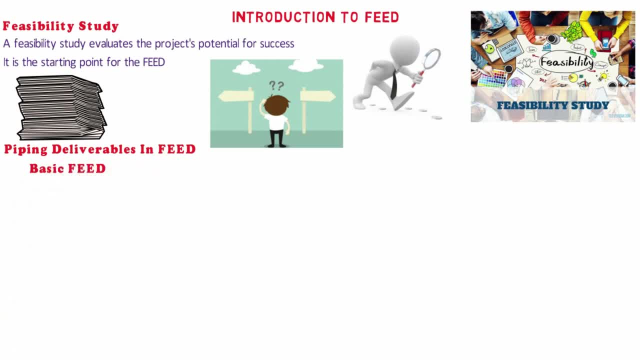 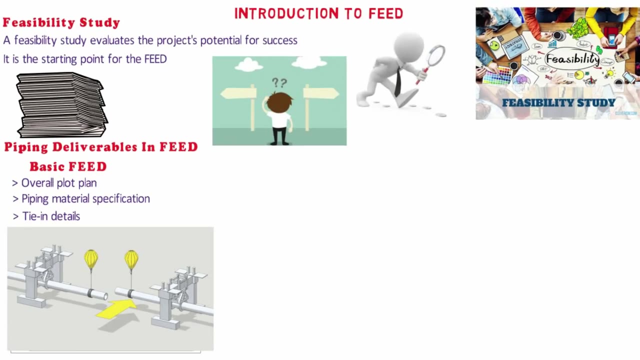 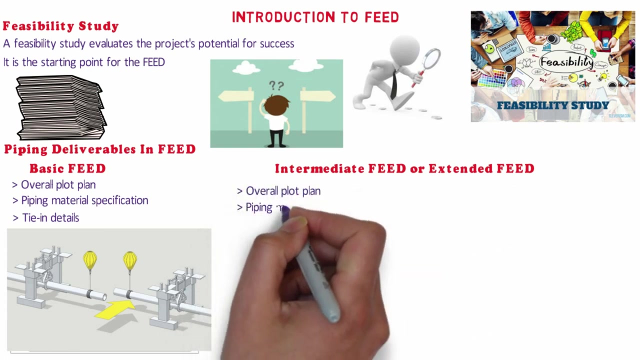 We can see like if we go for the basic feed We need overall plot plan Pipping material specification. So normally we have to give only brief description, tie in details and deliverable requirement for the intermediate or extended feed like overall plot plan piping material specification. 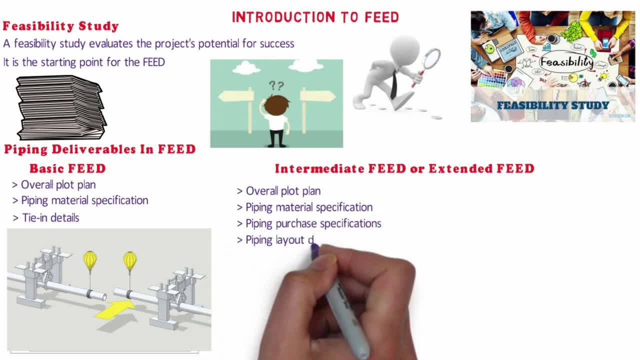 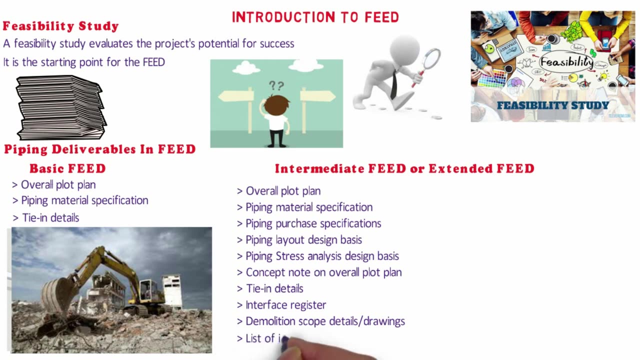 piping purchase specification. piping layout: design basis. piping stress analysis. design basis, concept. note on overall plot plan. Tie in details: Interface register, demolition scope and detailed drawings. List of important assumptions. Basis upon which the design is based. Extent of engineering carried out at feed stage. 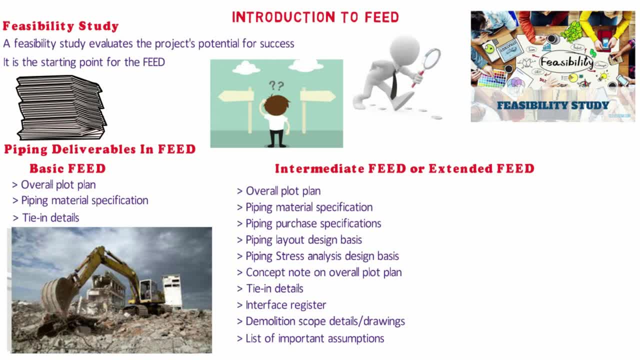 Outlining major engineering challenges or issues that need to be resolved during detailed engineering. for extended feed, One or many of the following additional deliverables may be required, if specific in the contract. The first one is the delivery of the feed. The second one is the delivery of the feed. 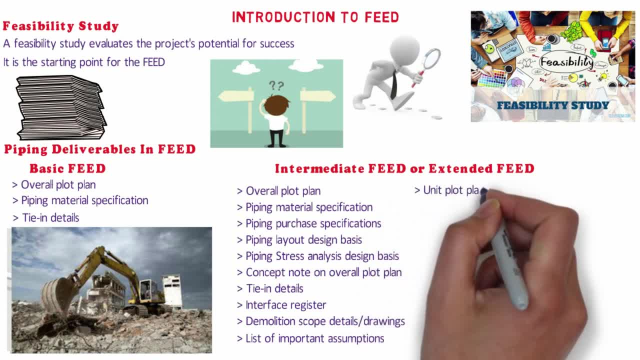 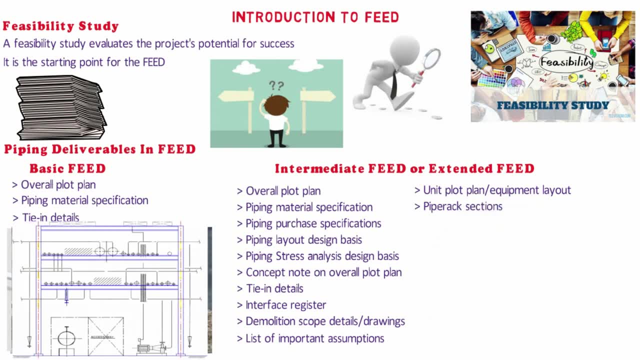 The third one is the delivery of the feed. The fourth one is the delivery of the feed. And finally, more usefulyu, will help more difficult applications likeê Unit plot plan or equipment layout, Piperec sections. For piperec and flat plot plan we have already prepared a video. 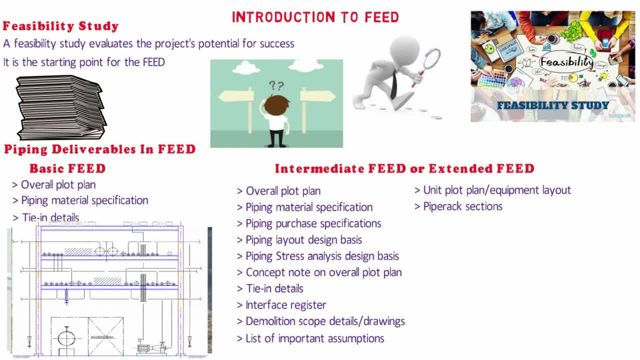 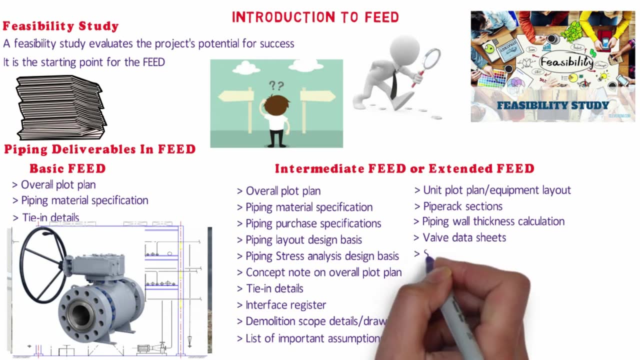 You can see in the above shared link or you can check in the description box below: Pipe wall thickness calculation. for this also We have prepared the video. You can check in the description box. wall datasheet. Special item lists- LISA. 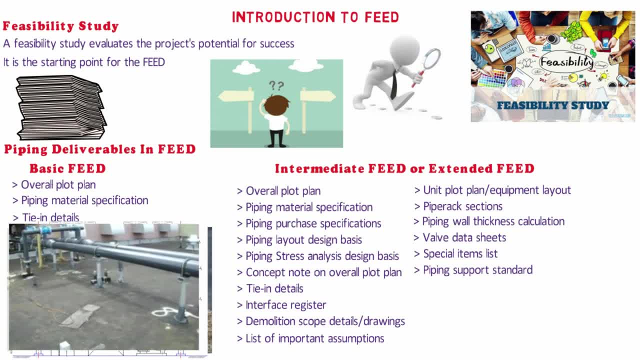 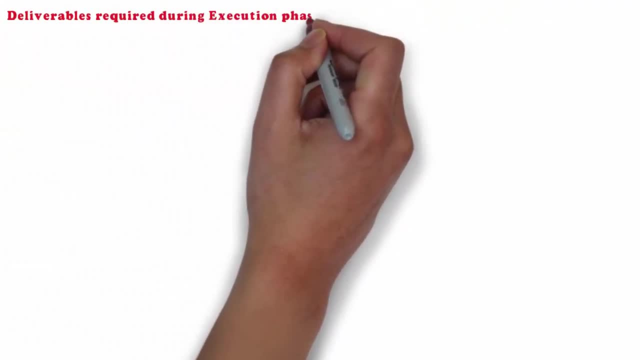 support standards. piping standard assembly drawings. piping GA for critical area and critical lines: only ITT package scope of work with respect to piping For execution phase. these are the deliverables required, like 3D model, up to 30% stage material. 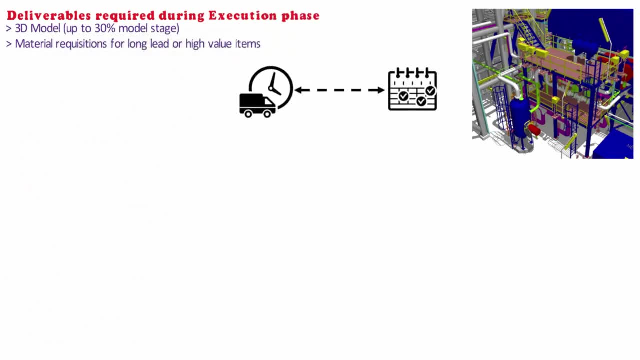 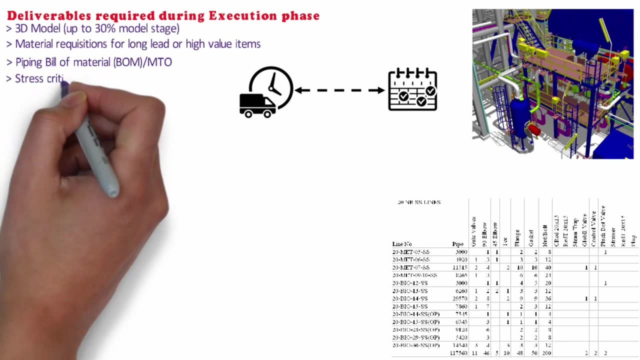 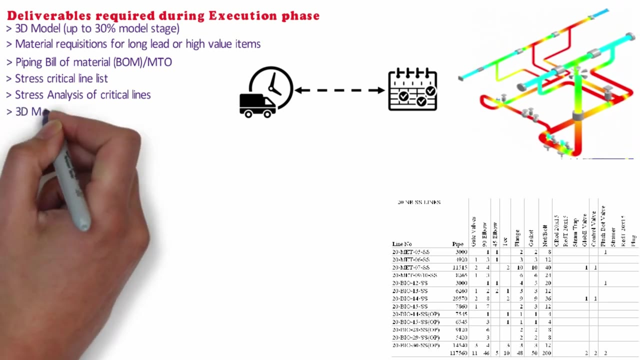 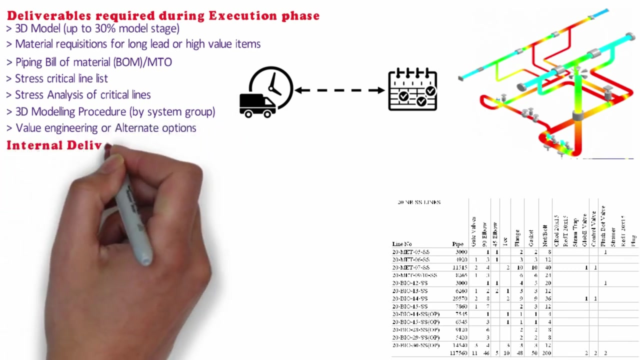 requisition for long lead item or high value item, piping bill of material, BOM or MTO. stress critical line list. stress analysis of critical lines, 3D modeling procedure by system, group, value engineering or alternate option. Some of the deliverables are required for the interdiscipline, which are like bill number. 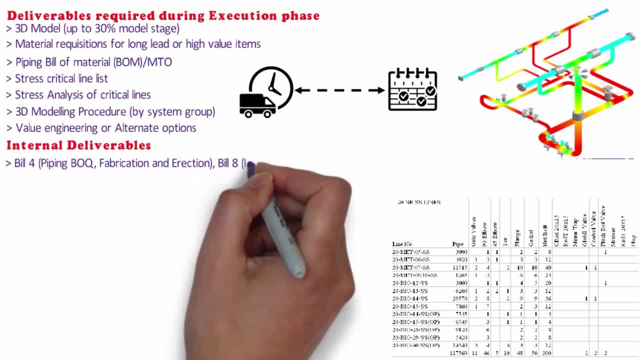 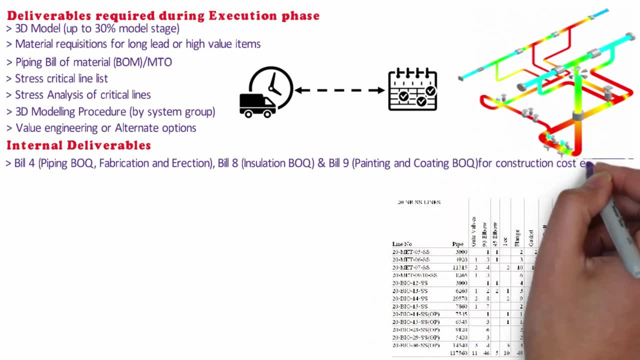 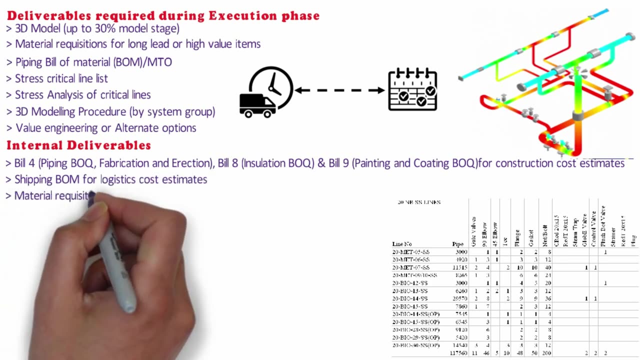 4. These include the piping BOQ fabrication and erection, bill number 8,. insulation BOQ and bill number 9, painting and coating BOQ for construction cost estimation. shipping bill of material for logistic cost estimates. material requisition if required for obtaining 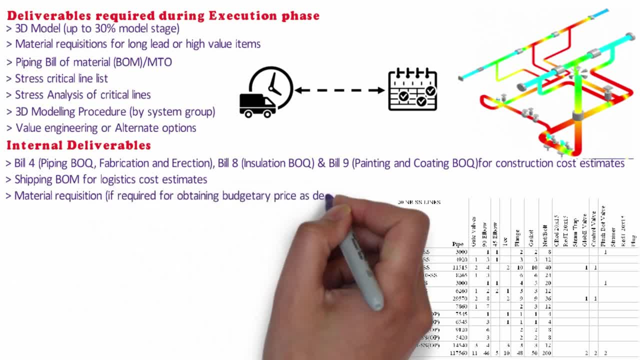 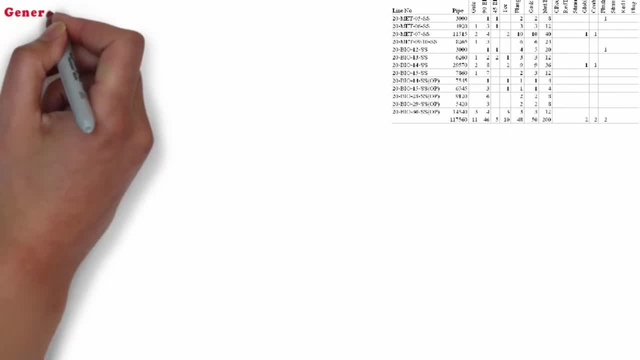 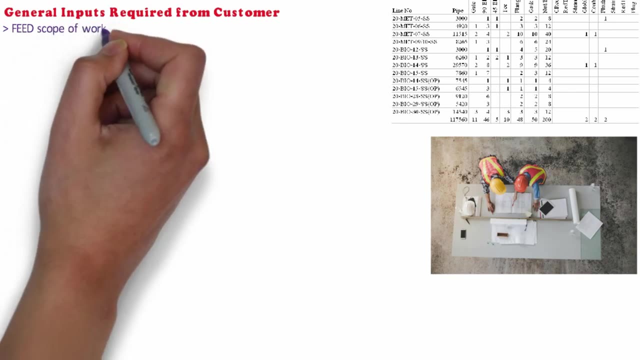 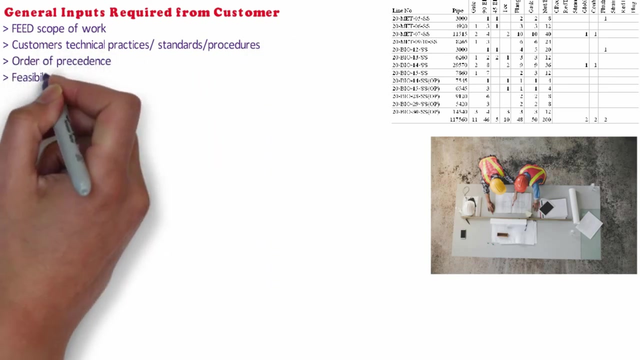 budgetary price as decided by proposal group, Cost estimate and cost basis. let's see what are the general inputs required from the customer to proceed. the feed one is the feed. scope of work, customer technical practice, standard procedures, order of precedence, feasibility study report, location and detail. 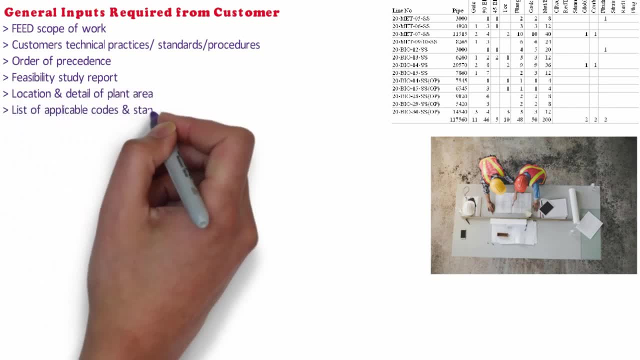 of plant area, list of applicable codes and standard with addition. So what things? normally? client reviews following reviews are generally carried out with the customer during feed. The comments shall be recorded formally in form of report, And same shall be incorporated before issuing the document which we already mentioned. like 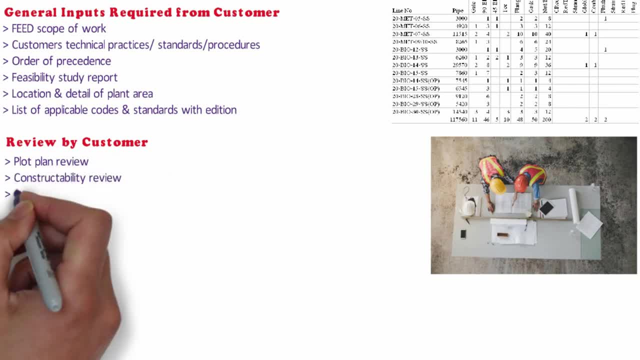 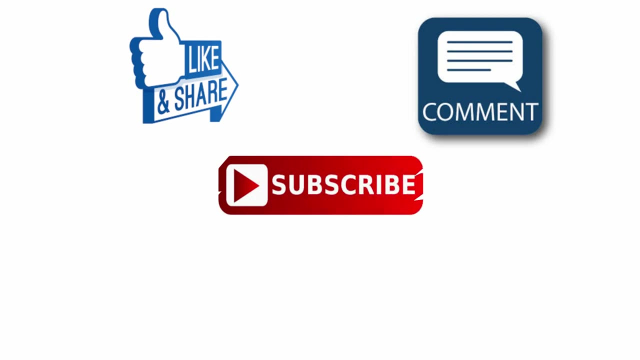 plot plan review, constructability review, design basis and specification review, 3D model review. as I said, 30% model review. So this is it, guys. hope you like the video. if you like it, please hit the like button, share, subscribe and keep helping us and let us know on which topic you want us to prepare. a video. thank you, have a nice day. 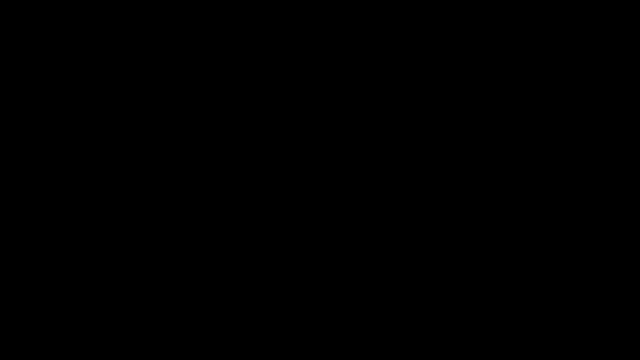 In this video we're going to talk about relative velocity. So when you hear the word relative velocity, what do you think of? What I think of? you're talking about the velocity of an object relative to something else, And whenever you want to calculate the relative velocity, it's basically the difference between two velocities.